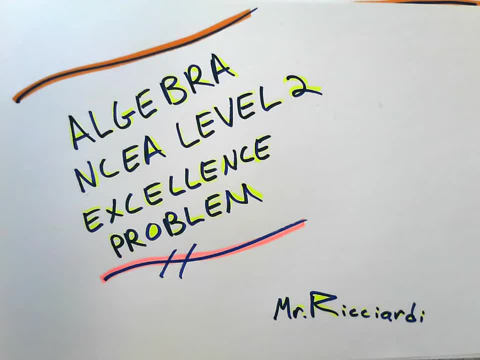 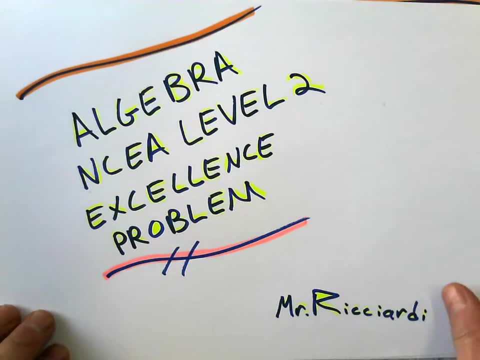 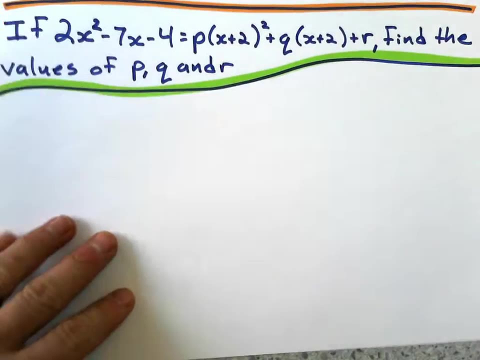 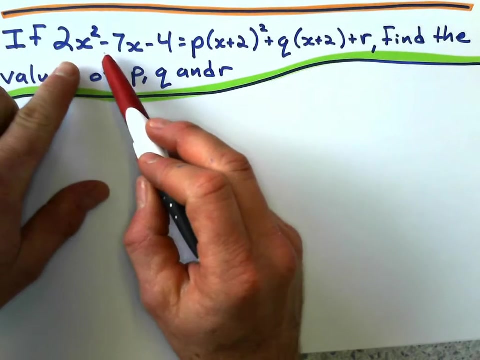 All right, greetings. Today I'm going to do an algebra level 2 excellence problem that I found and it's a pretty tough one, so hopefully I can walk you through it and make some sense out of it. Here it is, and we've got quite an interesting equation there. So if 2x squared minus 7x minus. 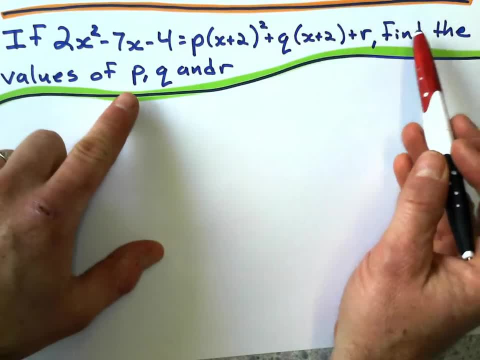 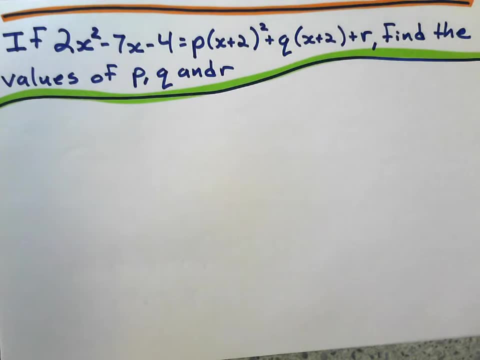 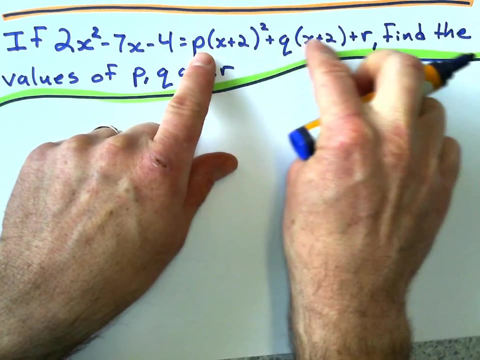 4 equals this expression. here we want to find the values of p, q and r. All right, now that looks pretty daunting. so I think how I first tackled this one is: I just kind of looked at this over here and I thought, well, maybe I can clean this expression up a little bit by expanding these. 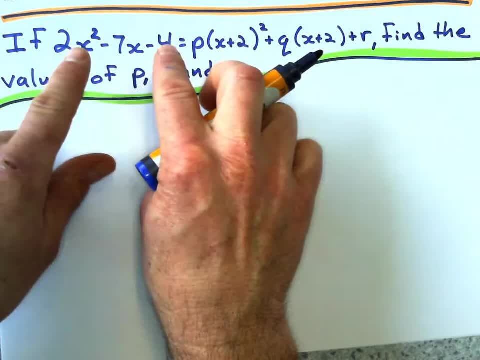 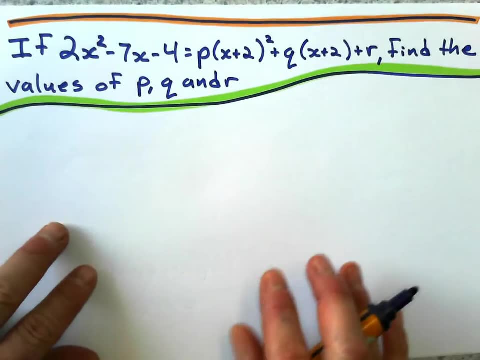 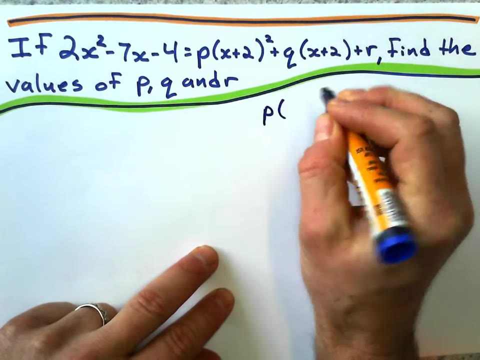 brackets and collecting any like terms, and then I'm going to kind of match it to this expression and then slowly solve for p, q and r. So here's what I did. First of all, I expanded these through, So I went okay, p, let's see. 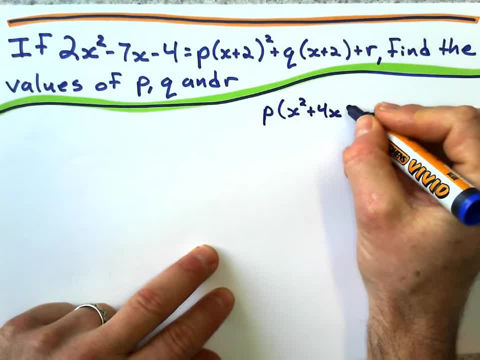 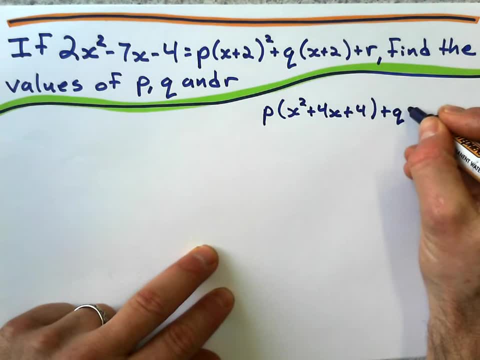 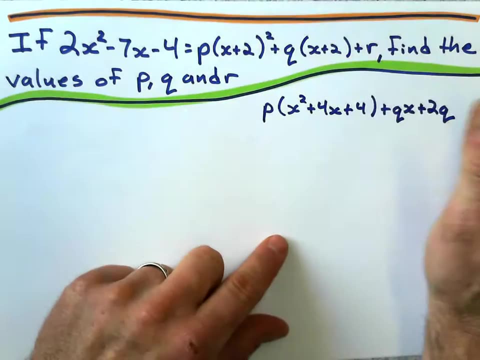 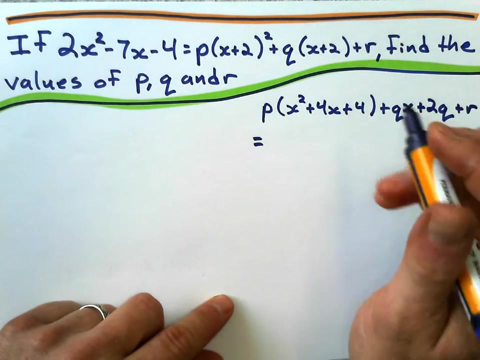 this gives me x squared plus 4x plus 4.. Okay, so that's that part. I expanded this part. I got qx plus 2q right there and then just a plus a power on the end. Okay, and now I just expanded that p through. 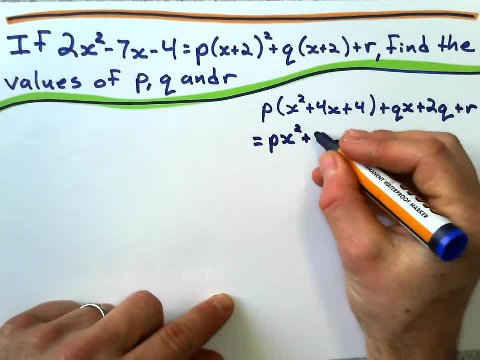 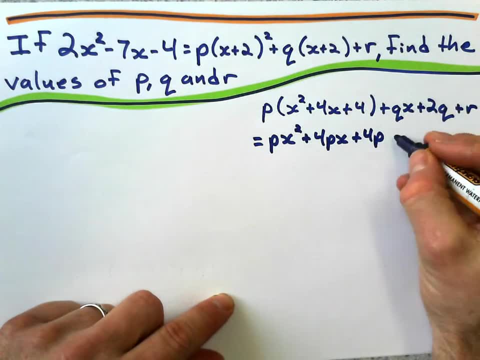 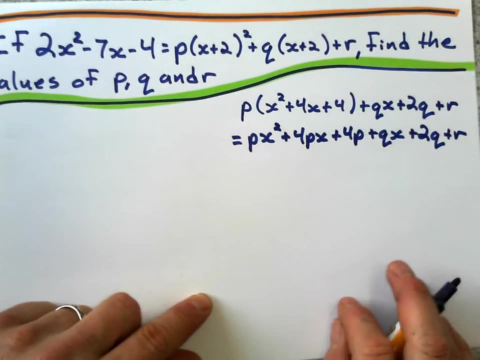 Again px squared plus 4px plus 4p, and then I just have all this stuff on at the end still and I'm going to clean up in a bit: plus qx plus 2q plus r. All right, let's fix that adjustment up a little bit. 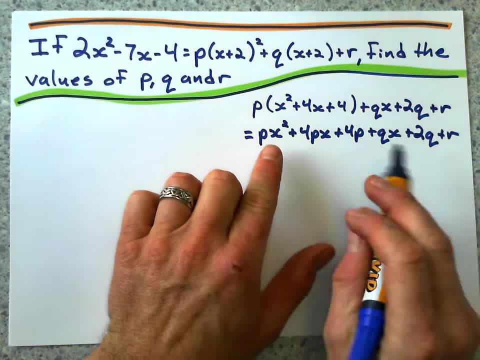 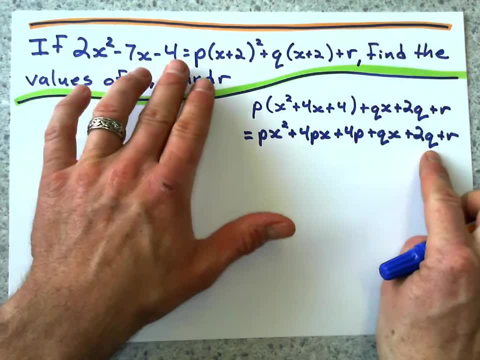 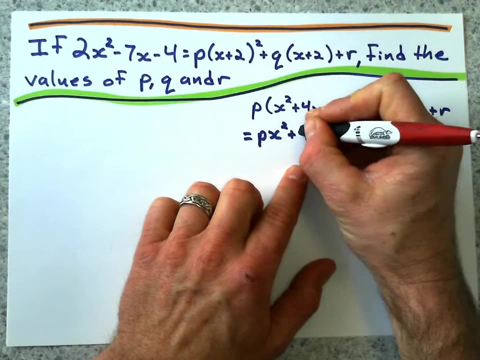 Okay, now from here, I'm looking at it and I want to make this expression look like this expression. So write the x squared terms first, any x terms next and any constant terms at the end. Now this looks kind of weird, but I'm going to try to say that these guys and these guys are like terms. 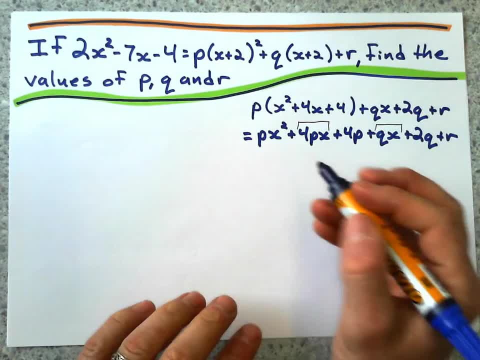 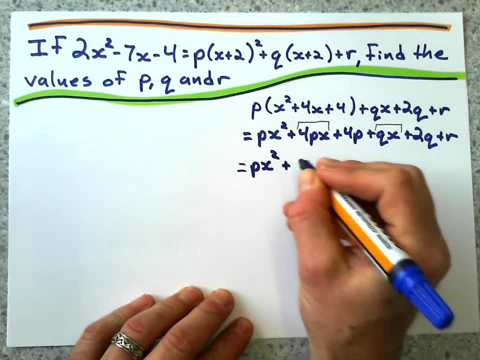 because they both have an x at the end and I can just say that the 4p and the q are coefficients. So I'm going to write it like this: I'm going to say that it's px squared plus. I'm just going to: when I combine them like this, I'm just going to combine their coefficients. 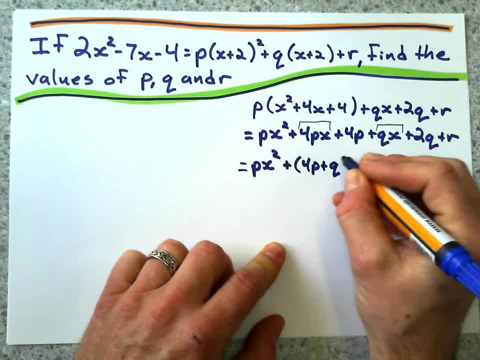 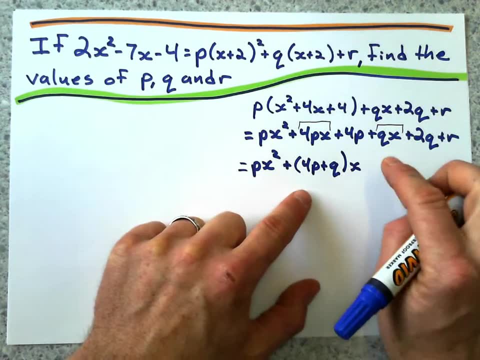 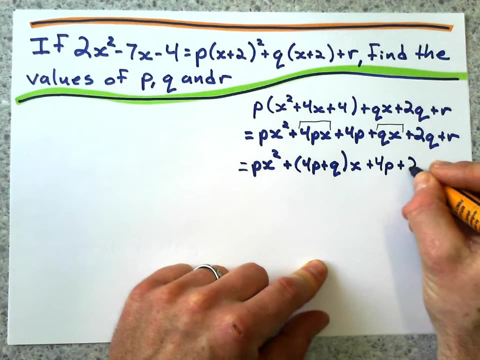 So this is 4p plus q. Now, I can't combine those because they're not like terms. Okay, so I just did that right there. Now everything else is just kind of what I wrote on the end. 4p equals 2q plus r. 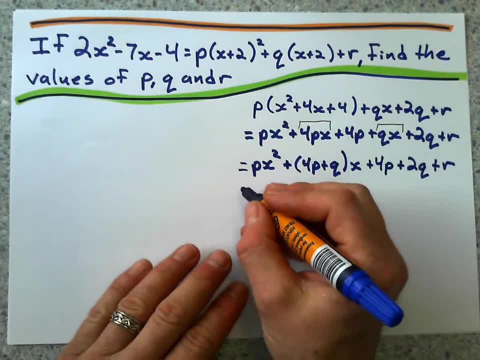 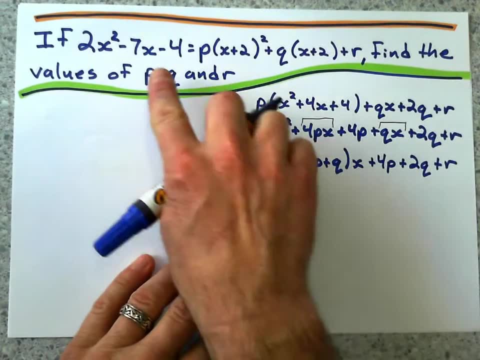 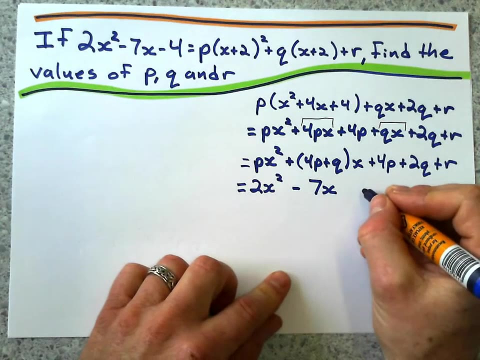 Okay, now what? Now? here's the interesting part. Now it says that this expression equals this first one. So that means that this big long thing right here must equal 2x squared minus 7x minus 4.. And I'll show you why I spread those out in a minute. 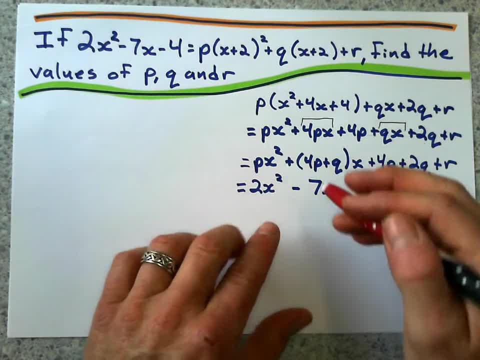 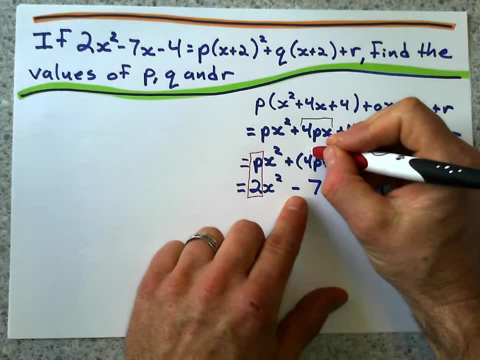 Okay, so these two expressions have to equal each other. Well, what that means is that I'm looking at these coefficients. Okay, t, It's got to be equal to 2.. And this expression- and I get this coefficient here- for p plus q. 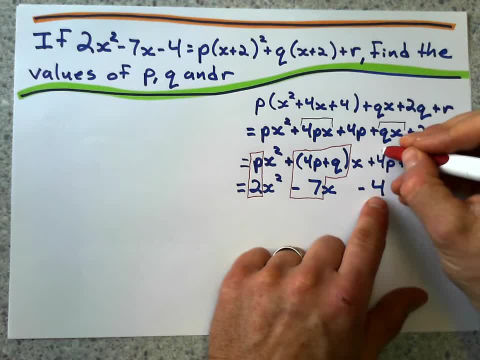 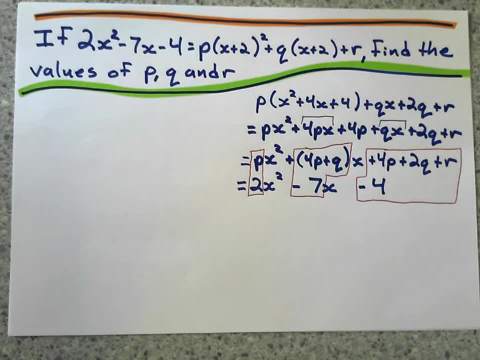 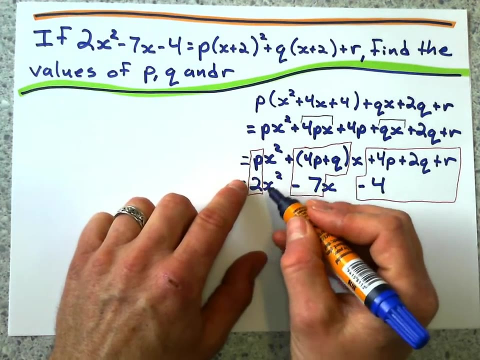 Well, that's going to equal negative 7.. And then all of this leftover stuff here is going to have to equal negative 4.. Okay, so that seems pretty daunting at first, But let's just take this slowly. Okay, well, I know p has got to equal 2.. 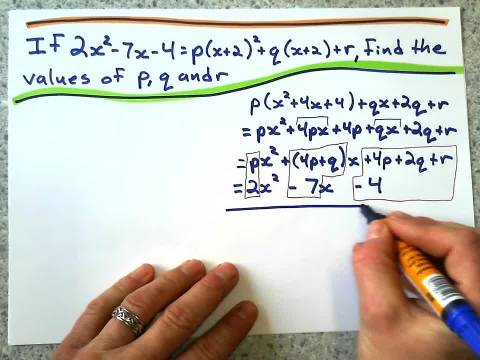 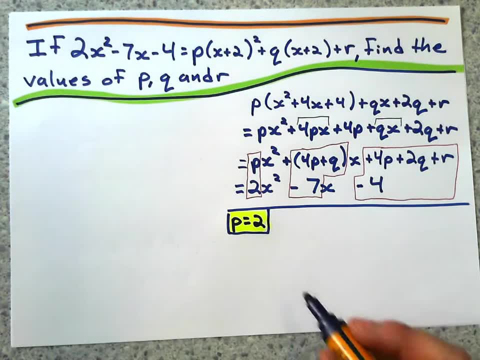 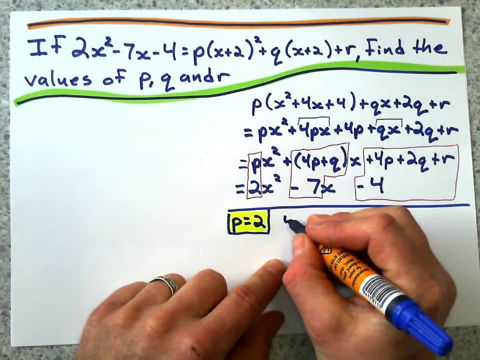 Because if px squared equals 2x squared, Then p equals 2.. So let's say, okay, so p equals 2.. That's done Now. what happens next is kind of like a chain reaction solving here. So if p equals 2, that means that I'm going to substitute it into here. 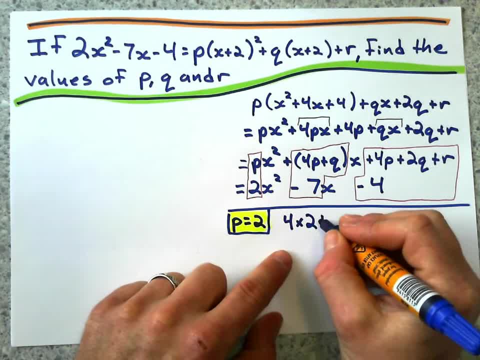 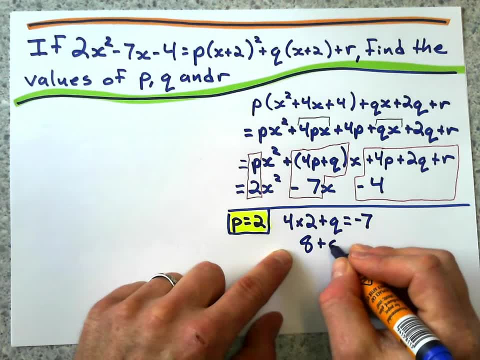 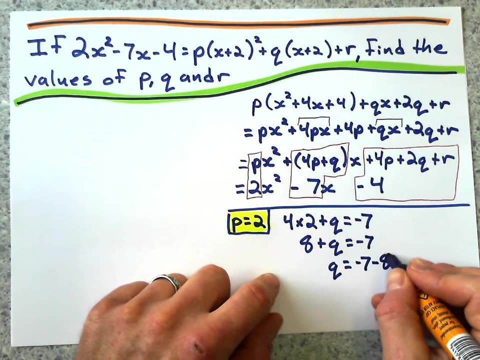 And that means that 4 times 2,, which is p plus q, has got to equal that negative 7.. 4 times 2 is 8.. 8 plus q is negative 7. That means that q must be negative 7 minus that 8.. 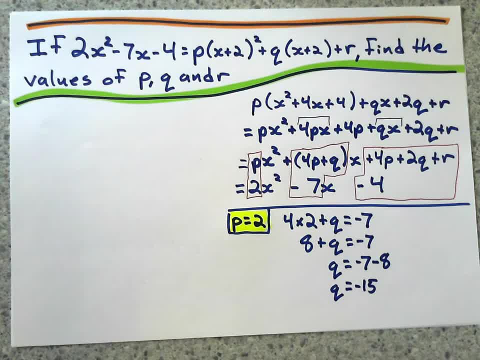 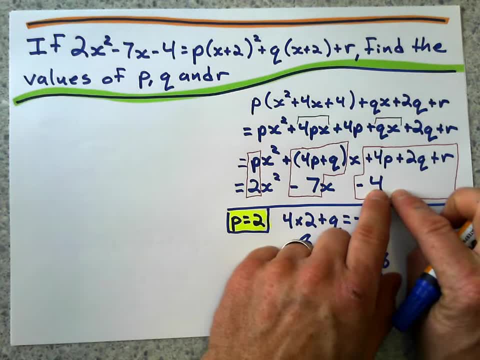 That means that q must equal negative 15.. Okay, now I'm getting somewhere. Okay, now for the last part. I've got this big expression here: that's going to equal negative 4.. Okay, and I've only got p and q. 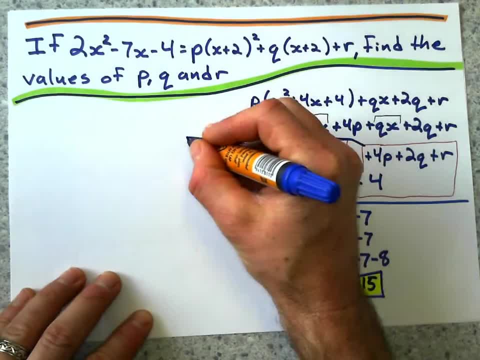 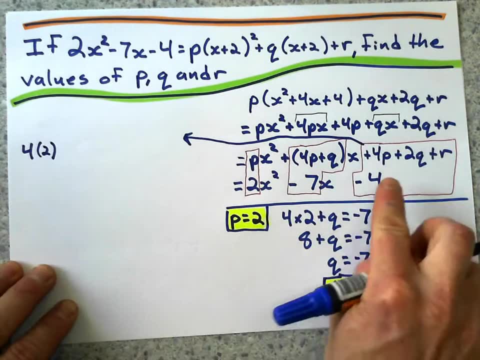 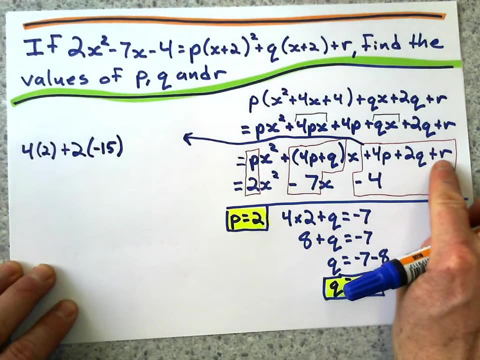 So I'll get the bodies of p, So I'm just going to kind of put this over here. Well, this means that 4 times the value of p, 4 times the value of p, which is 2,, plus 2 times the value of q, which is negative, 15.. 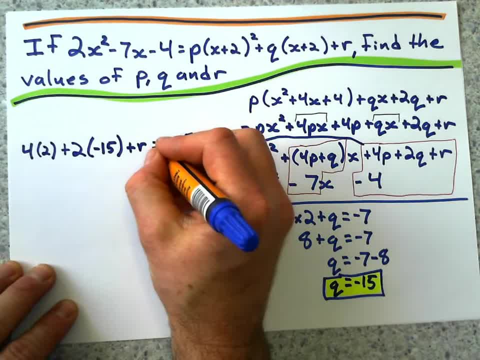 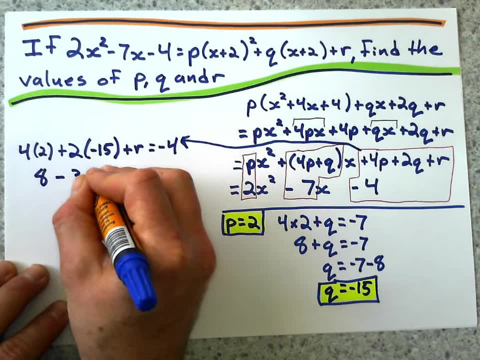 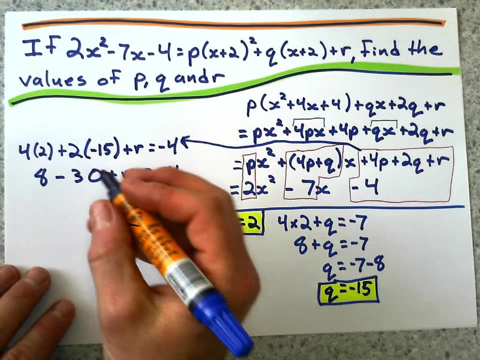 Where am I? Plus r has to equal that negative 4.. And I simplify this a little bit: 8 minus 30. plus r equals negative 4.. 8 minus 30, what does that give me? Negative 22.. Plus r is negative 4.. 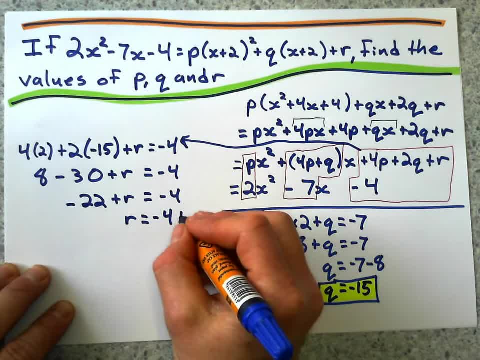 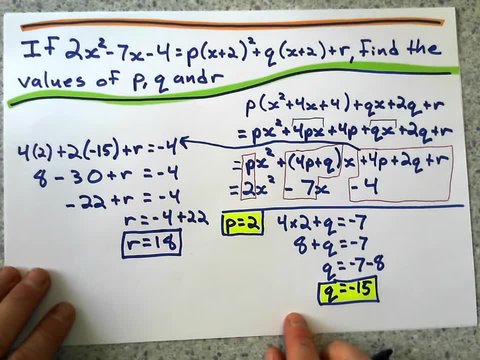 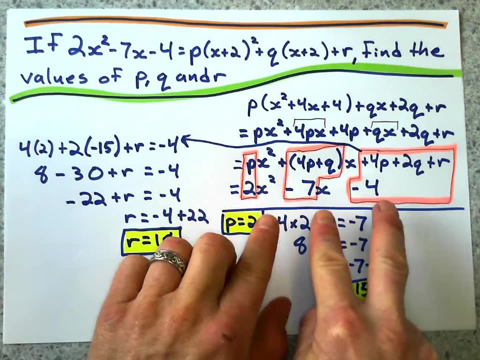 So that means r. when I add 22 to the other side, I get a value of 18.. Okay, now, that's a hard problem to do, And I think the hard part is knowing to set these two expressions equal to each other. 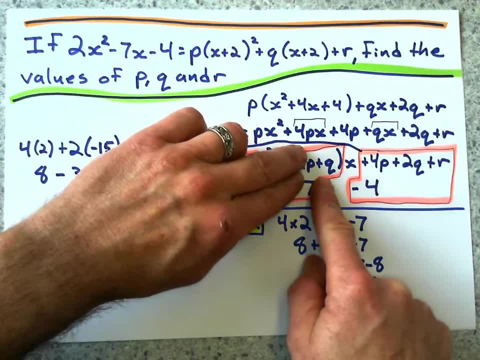 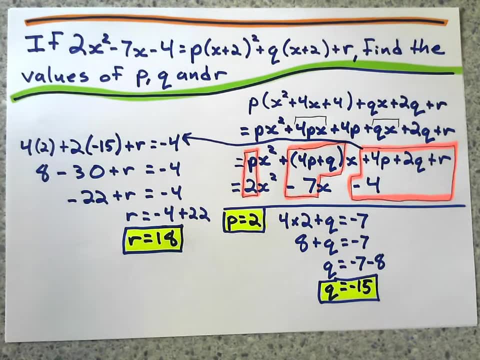 And we're just solving for those coefficients. And once we get p, well then we can get q. Once we get q, well then we can get q. Once we get q, well then we can get i. And so, yeah, it's a hard problem, but there it is.